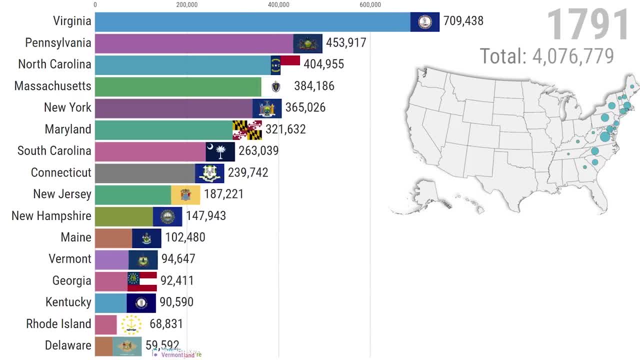 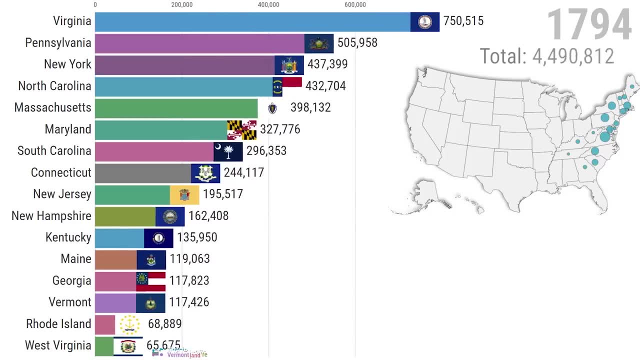 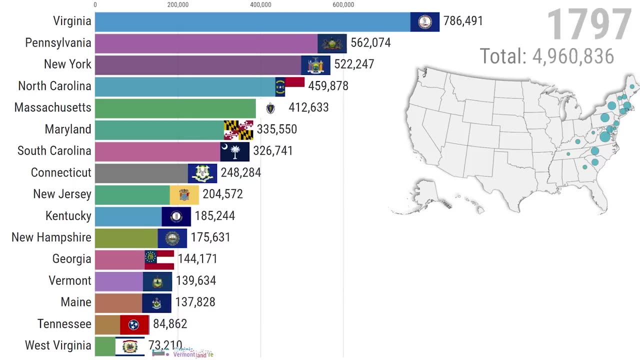 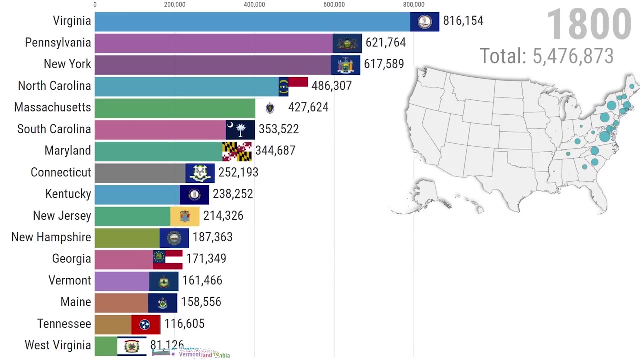 This video is a derivative work of the project. You can watch it in the following video. The first video is a video of the foundation of the church. The second video is a video of the church building. The third video is a video of the. Thank you. 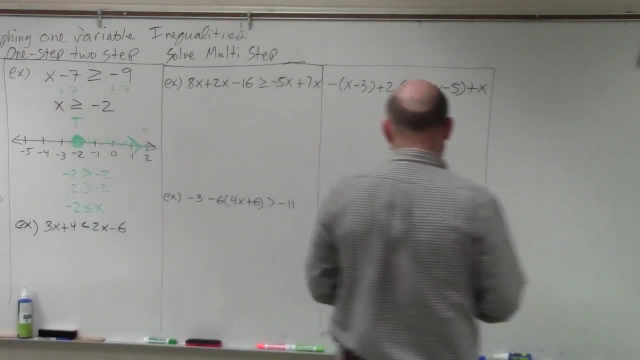 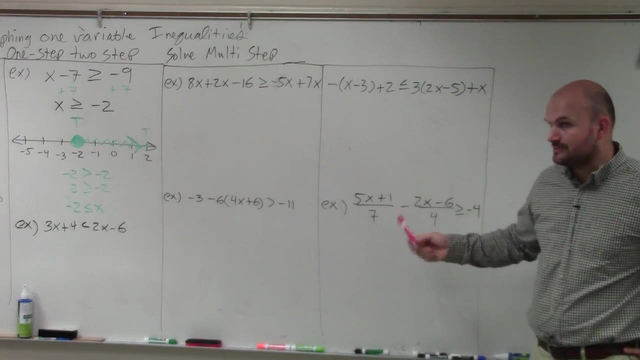 When you guys have a problem with the fractions, again, the process is going to be exactly the same, But in this example we got to simplify. Well, we can't combine like terms because if you guys remember fractions, you can't combine fractions when they have common denominators. 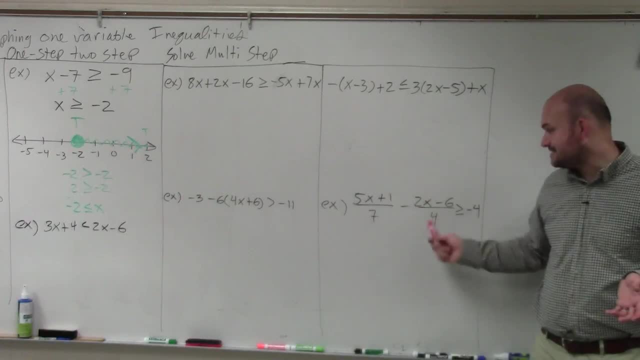 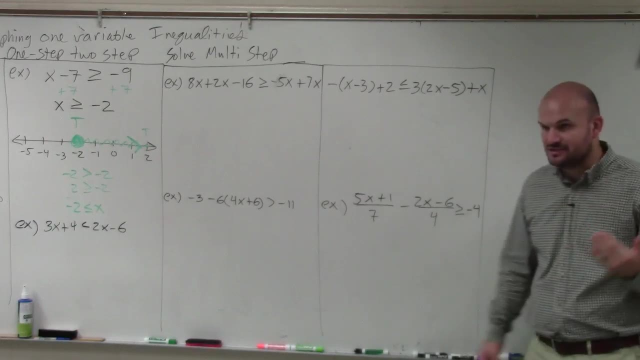 right, So I can't combine these. If they have the same denominator, then I could simply combine them, But anyways, I don't even like fractions. anyhow, I want to get rid of fractions. I don't like fractions at all. So the best way to get rid of fractions, like how we did on that one example: 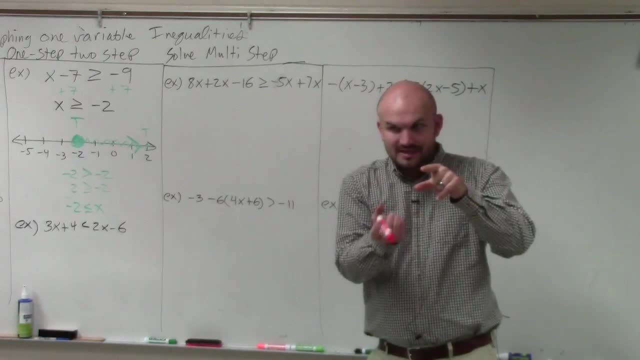 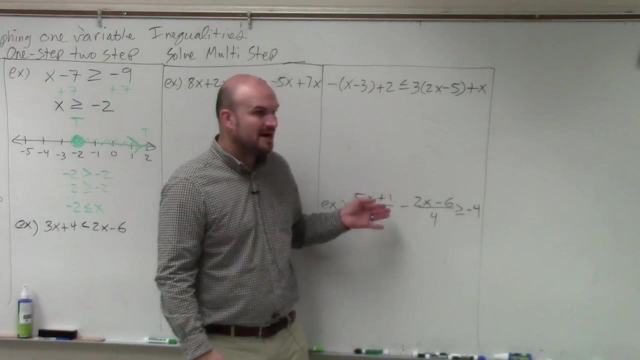 remember we had r divided by 20.. 20 was in the denominator. To get rid of 20, we multiply by 20.. Well, here we have different denominators, So we don't want to multiply by 4 and then multiply by. 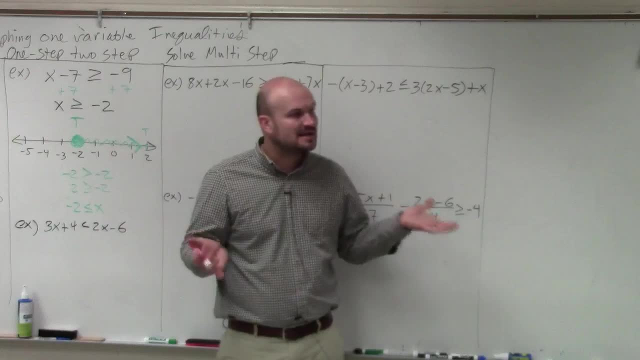 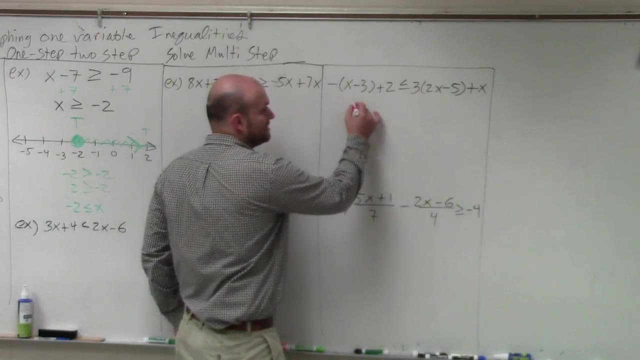 7.. But what we do want to do is multiply by the common denominator, what we call the least common denominator. So we want to find the smallest number that 7 and 4 both divide into. So to find that number we can just list the multiple: 7,, 14,, 21,, 28,, 35.. 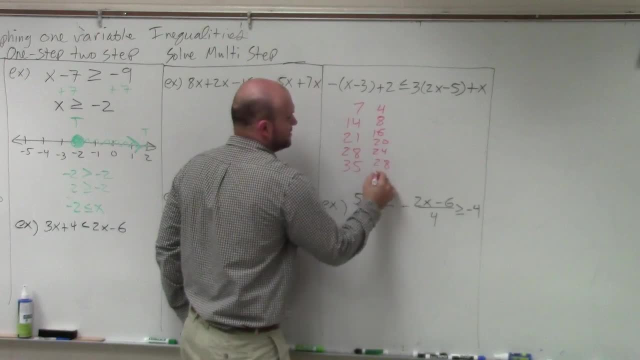 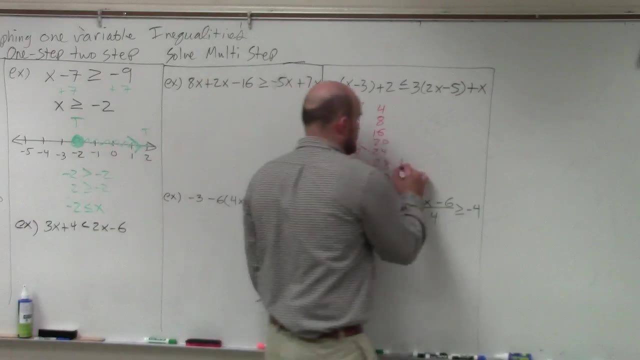 4,, 8,, 16,, 20,, 24,, 28,, 32.. And what you guys see is the smallest number that both 7 and 4 divide into is 28.. That is what we call our least common denominator, our least common multiple. What? 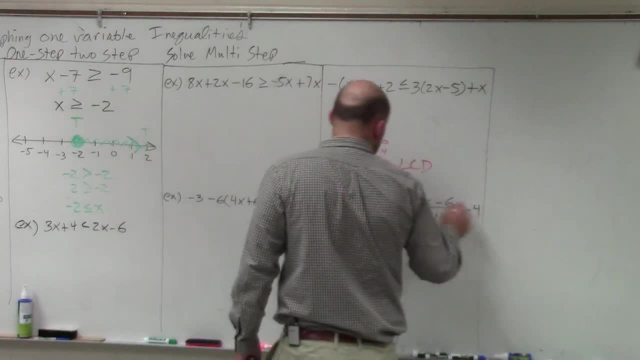 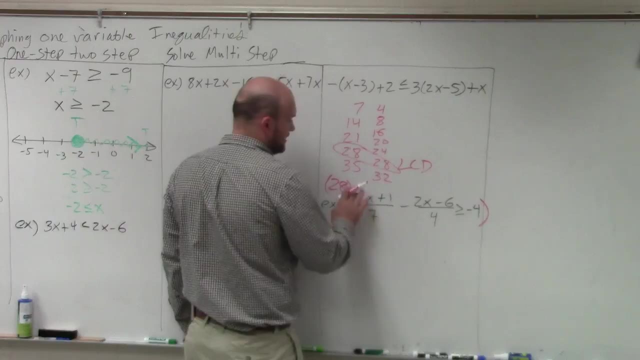 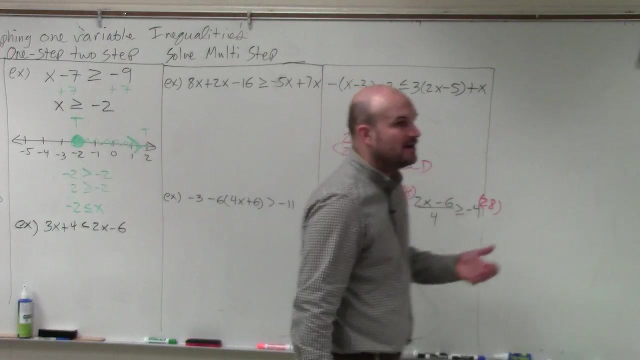 you're going to want to do is multiply everything by 28.. Actually, I forget the parentheses, So let's multiply. You're going to want to multiply every single quantity times 28.. Now, the reason why we want to choose a number that 7 and 4 both divide into is because, rather